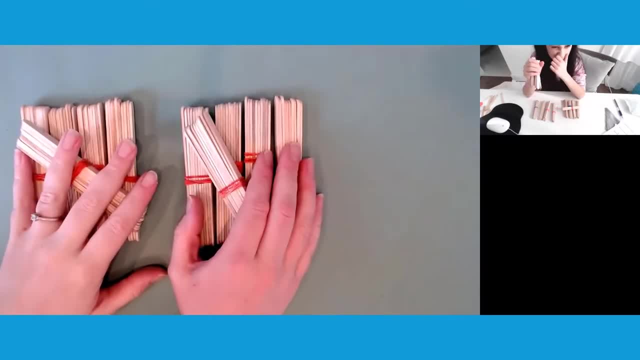 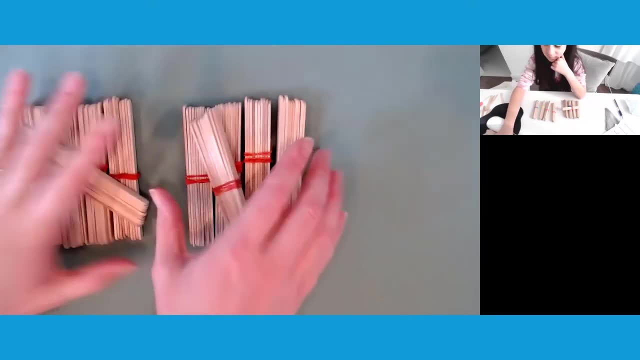 Yes, So when we have two fives in a place value, we have 10,, right, Yep? And so that would make a silly number. So anytime we have these two groups of five, we're going to bundle them up and make a 10.. 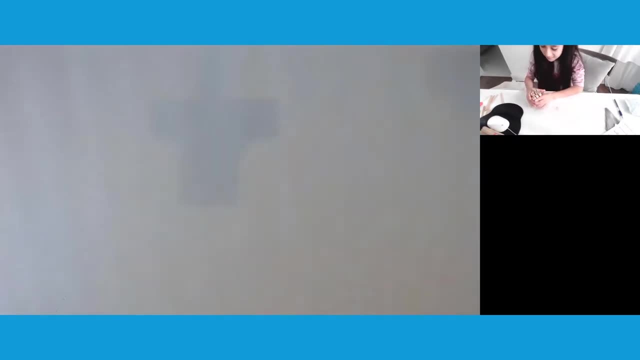 All right, But this is not a 10 anymore. We wouldn't leave this in the tens place. What is this now? A 10. A hundred? It's a hundred now, So we'd move it over to the hundreds place. 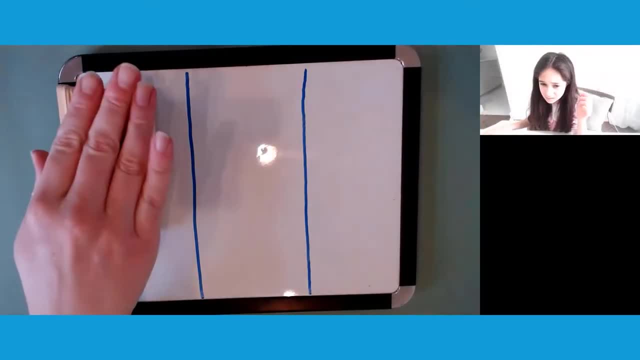 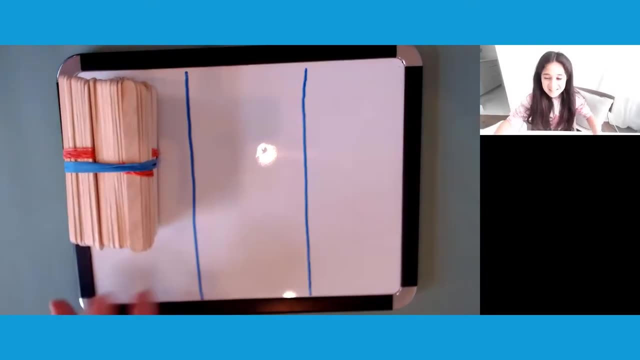 I forgot to bring rubber bands. Well, you don't have any more tens, do you? Oh, I have 10.. Oh, you do? Yes, Okay, But I said if I have another one of these then I couldn't do it. 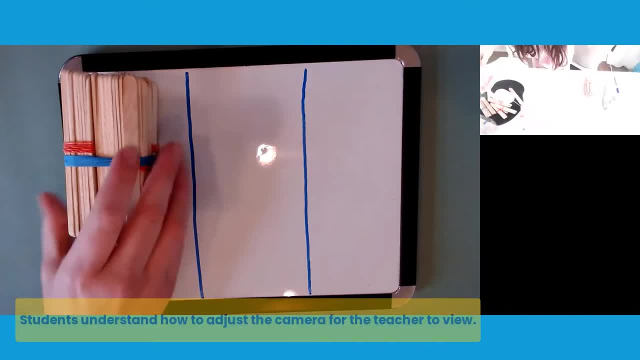 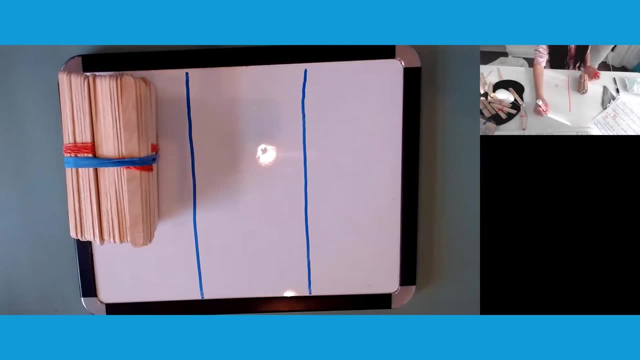 Yeah, Let's not make another one. Go ahead and hang on to that hundred and put it over here. I thought you meant that I was like what, Okay, So I'll do this? There you go, Good, Okay. 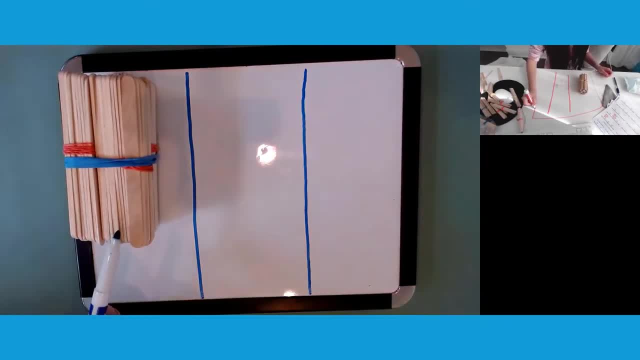 Okay, Your little box, because mine is a whiteboard table, not a whiteboard. Okay, All right. So what is this number made of? It's made out of 100 and zero. Okay, So it's made of 100.. How many tens? 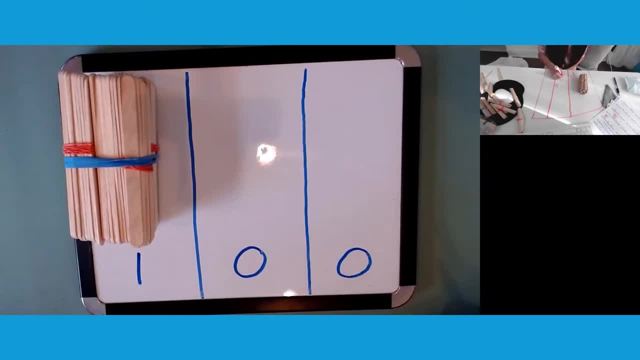 Zero, Zero, tens. And how many ones? Zero? Okay, What's its name? 100.. Good, Its name is 100.. Okay, Let's change this. Okay, How would we make this be 110?? Well, you're a fast racer. 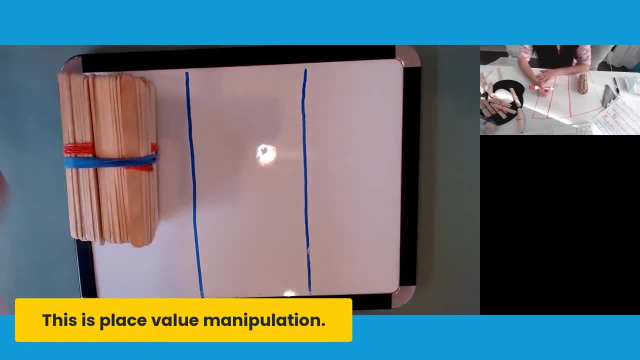 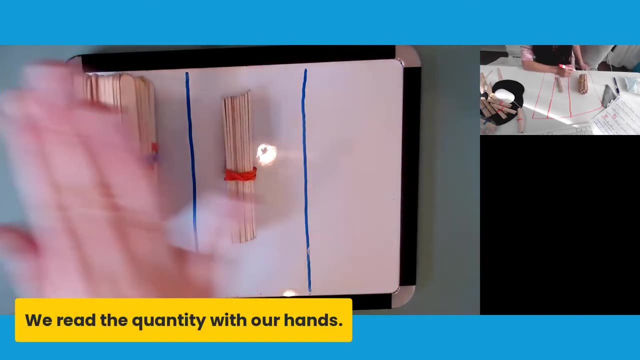 Lots of practice. How would we make this be 110? 110.. How do we do that? We would need another 10.. Oh, you're right. Okay, What's this number made of One, 100.. 100.. 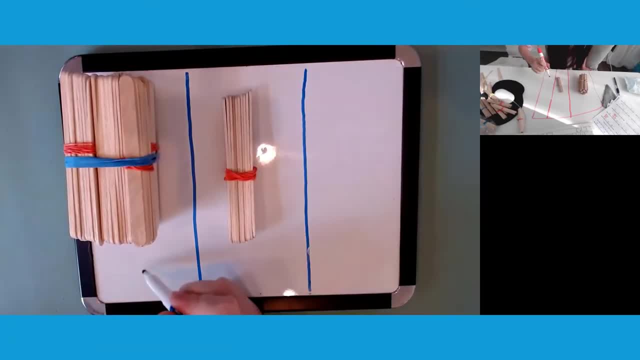 Okay, 100.. Yeah, that's its name as well. You're right. It's made of 100,, 110, and zero ones. Its name is 110.. Oh, this is a lot of tens. Look at all those tens in there. 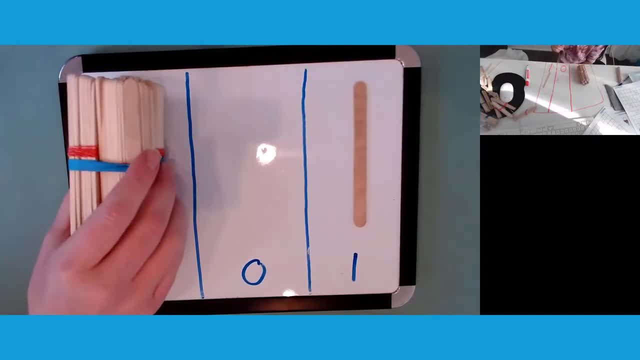 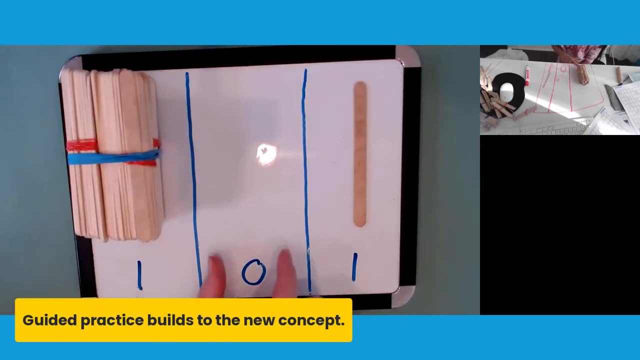 Oh yeah. So what is this number? This is 100.. Good And 10.. So it's made of 100.. How many tens? Zero, Zero tens, And 11. And 10. And one. 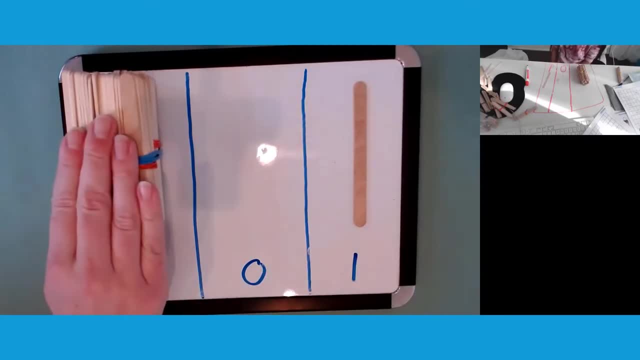 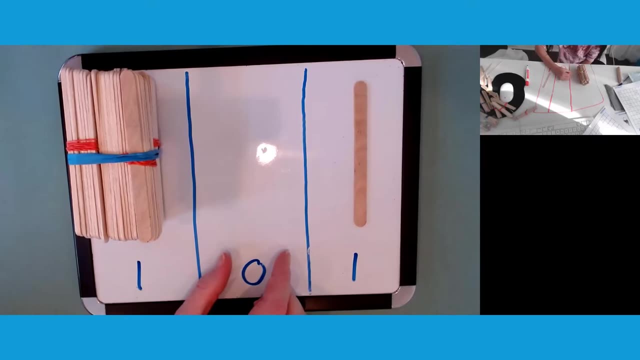 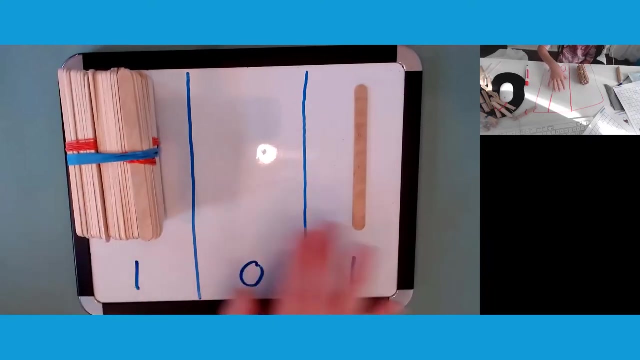 And one one. So one more time, It's made of 100, zero tens and one one. One one, ten and zero ones and one one one. Yep, 100, zero tens and one one. What's its name? 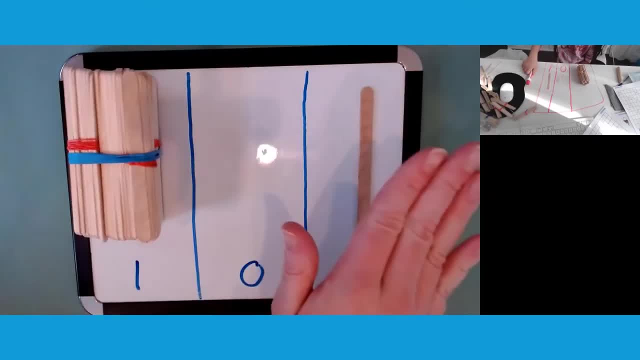 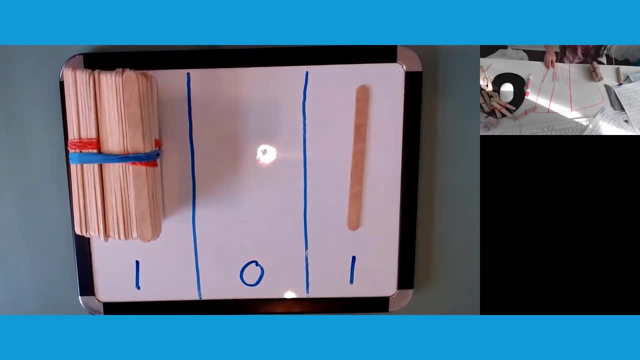 101.. Yes, 101.. Very good, If this is 101, can you make it 102?? Yes, Very good. Okay, What's its name? 102.. Good, 102.. Can you touch it while you say it? 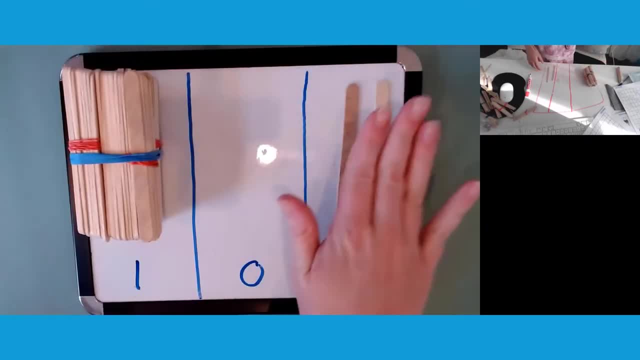 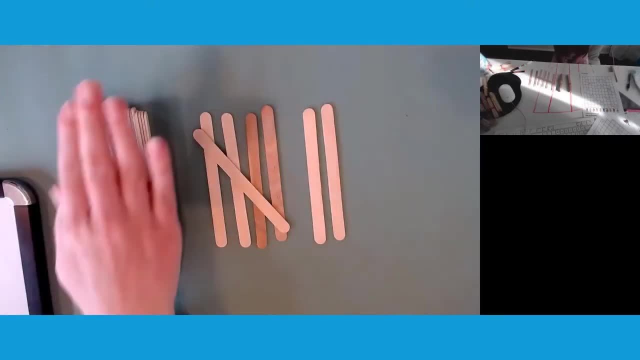 Yes, 102.. 102.. 102.. Good, 102.. Well done, Okay, I'm going to have tens. Good, So we have two. what Two? tens and seven ones, So that must be 27.. 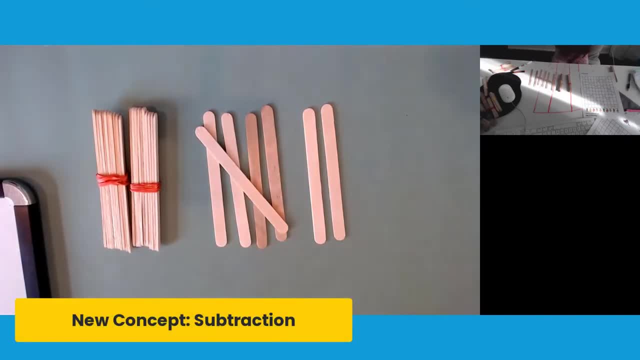 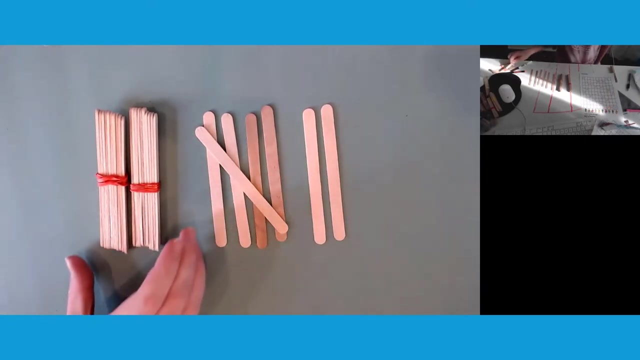 Good, Juliana, Nice work. If this is 27,, do you know how many tens it is? how to make it say 26? 26. How do you do that? Okay, so 26.. So let's look at this: 26. Which? 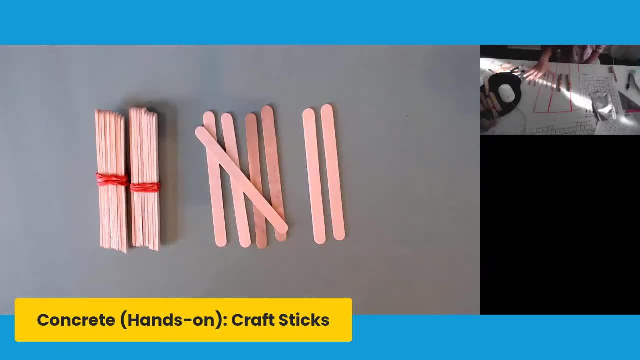 one is not right, Which one has to change This? Ah, this is not right. Okay, how do we make this? say six? Oh, not so fast. It's not quite as big of a change as you think. It's pretty small. 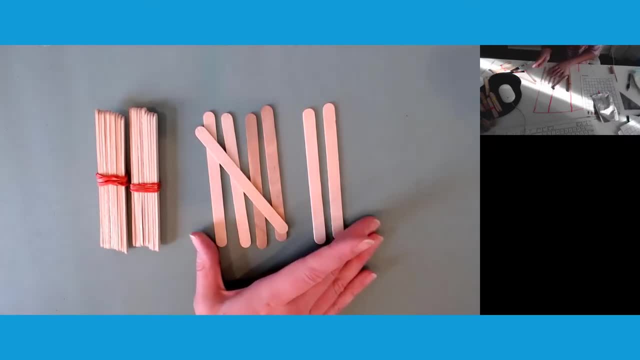 Really, Really. I liked your voice. That was funny, Really. All right, how do we make this say six, How do we do that? It's a small change. It's not as big as you think. Okay, What does? 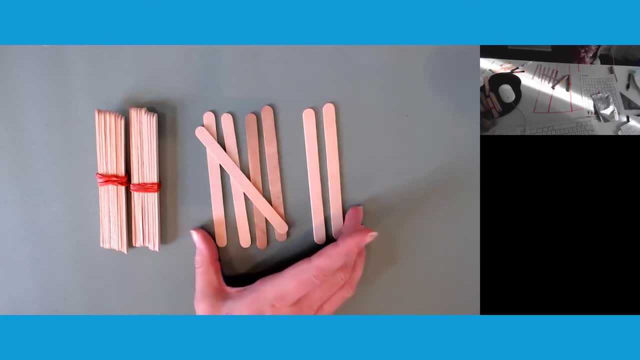 this say now It says 52. Let's see, here I can see why you're saying that These are all ones. How many ones are there? Ah, seven, There are seven. So how do we make this say six? 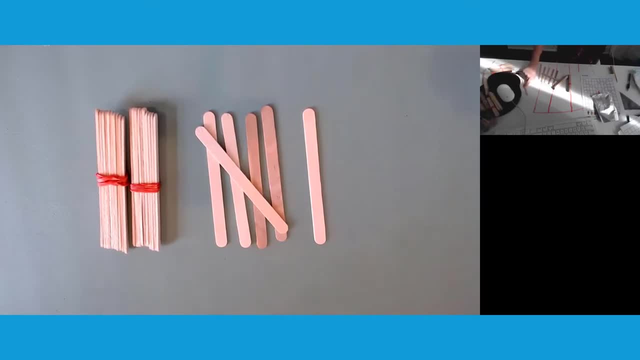 Oh, see, a very small change. Okay, what's this number made of? Made out of two tens and six ones. You're rocking it. What's its name? Its name is 26.. You got it, And I know, if we take away one it would be 25.. Oh man. 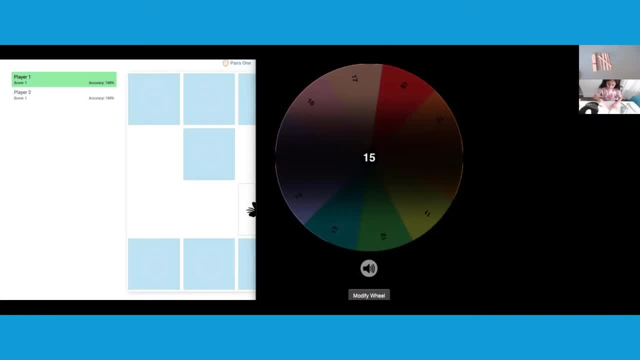 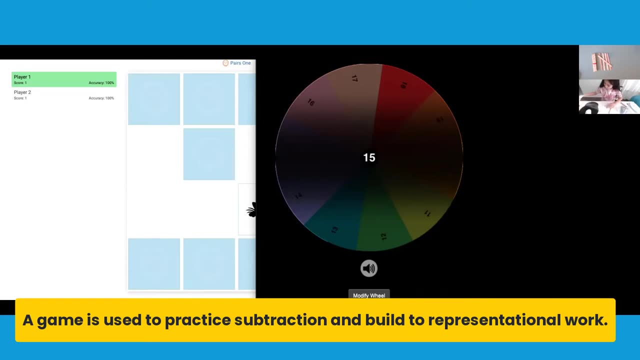 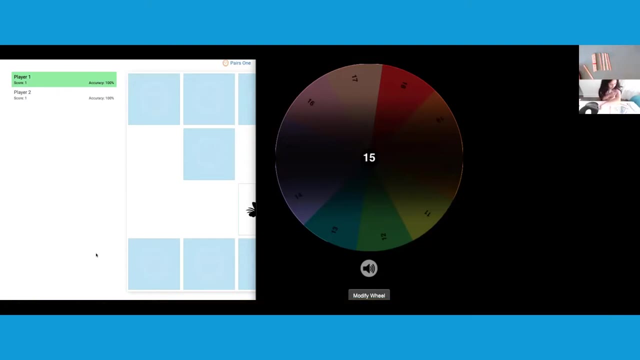 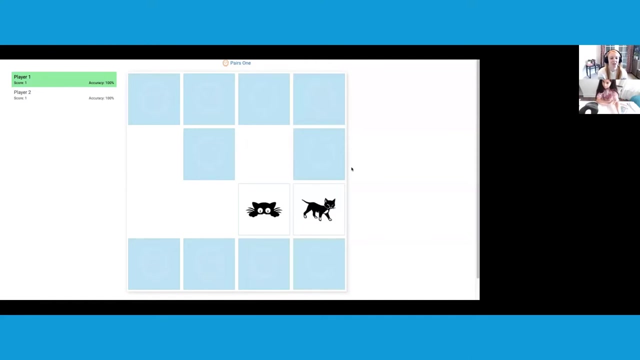 you're getting so good at this, You're on a roll. Okay, Take one away 14. 14.. Very good, All right, So let's go ahead and see if you can find a match. Okay, I bet you can. 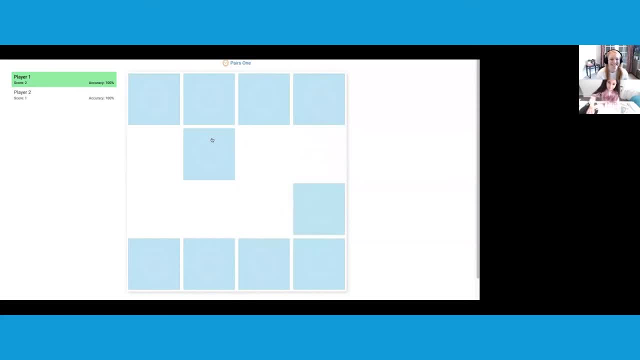 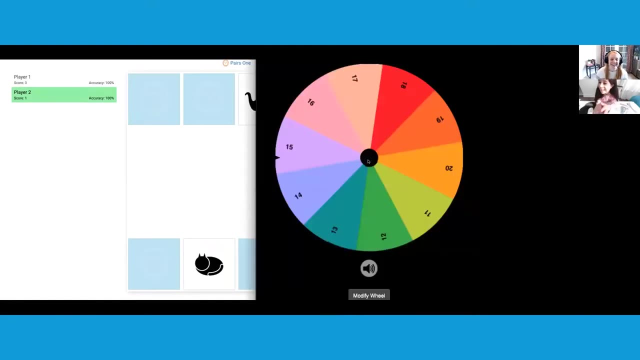 Oh it's so cute. Two matches- Oh it's so cute. I love the cute kitties. Oh, they're all so cute. Okay, I know he would just add to the cuteness, wouldn't he? Okay, 13. I'm. 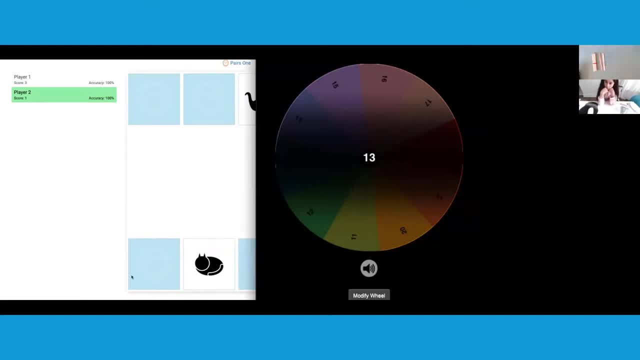 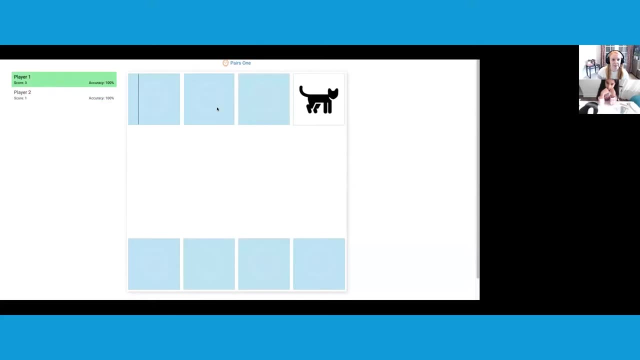 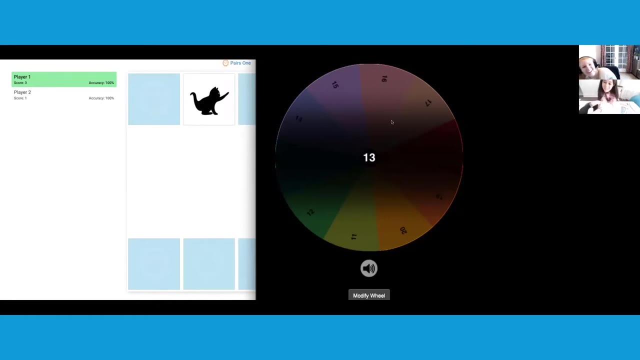 going to take one away, 12.. One less is 12.. Okay, Okay, See if I can find, I think you're going to find- another match. I think you're going to win. I hope you win. I hope you win. Okay, go ahead and spin. 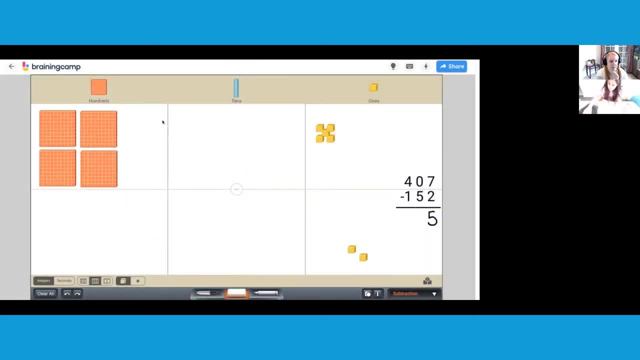 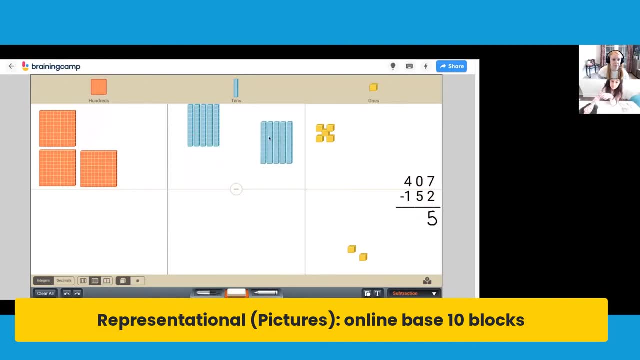 Okay, We need to take, we need, we need from the hundreds place to the tens place So we can get more stuff. Yeah, So now we have enough, but let's make sure we fix this up up here. Okay, This says we have four hundreds. Do we have four hundreds anymore? 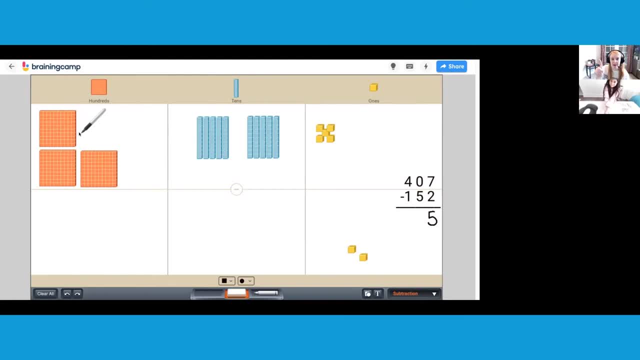 No, No, we took one away so that we'd have enough in the tens place. So how many hundreds do we have now? Three only, We only have three. So can you say: cross out the four and put a three, Cross out the four, put a three. 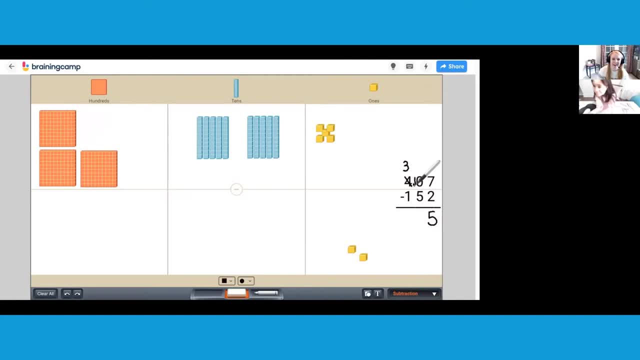 So one, I sound like a squeaky mouse Because we have 10 tens now, don't we? Yeah, we have 10 tens, There are 10 tens. Good job, All right, Juliana. what does the tens column tell us to do? 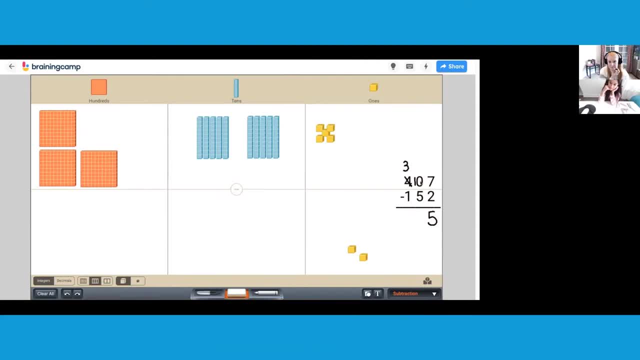 It says 10,. take away five. We have to take away five, Okay. So I think this is all five right. Oh, here, let's try. I mean that's all right. Can I have some help? Thank you for help. 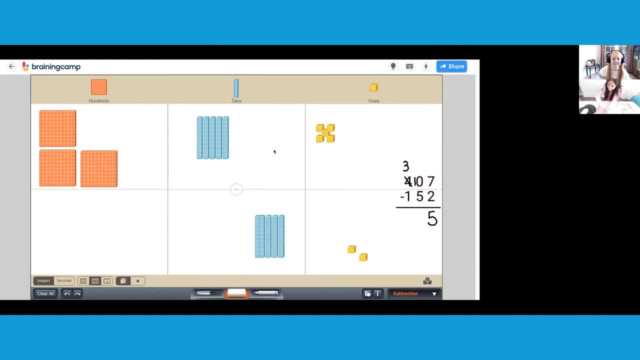 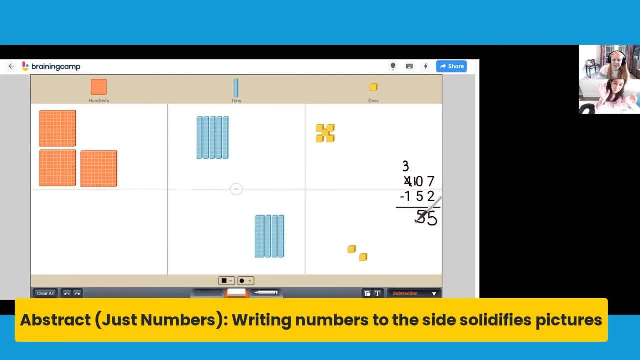 Oh, there it goes. Yay, Thank you. Okay, that's hard to move sometimes. You got it. Yep, I know I got it. Okay, that's five, Hooray, I just knew, because two fives makes 10.. 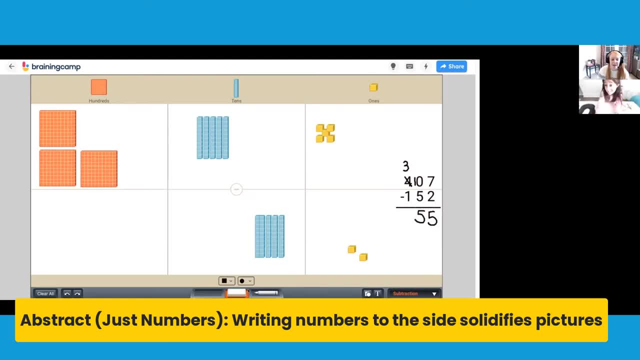 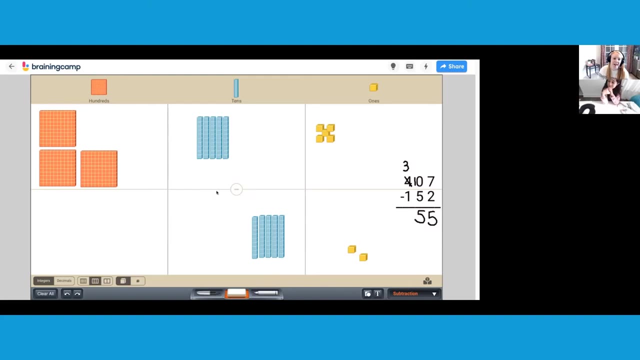 Mm. hmm, I mean hundreds. Okay, Well, two, Well, yeah, so two fives make a 10.. Two fifties or two fives made out of tens would make a hundred. Yeah, it's. it can take some practice understanding that. Okay. now, what place value do we need to take care of? 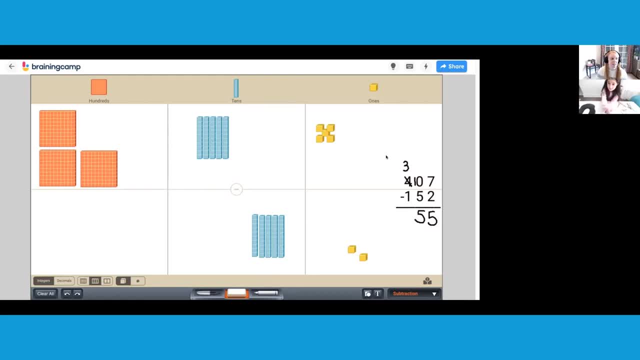 Now what? the ten hundredths place, The hundreds place Is to take away four. Okay, so we have three. I mean take away three, Three. It says we have three, Oops, three minus one. Take away one. Take away one. 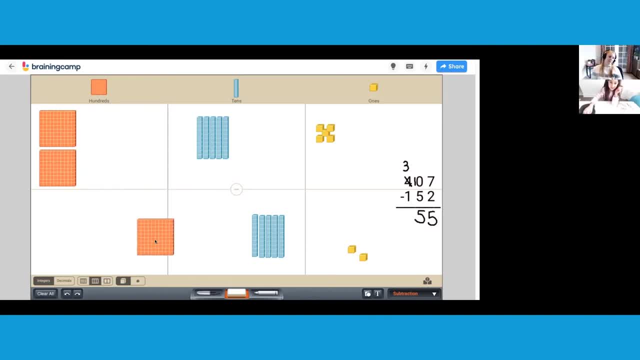 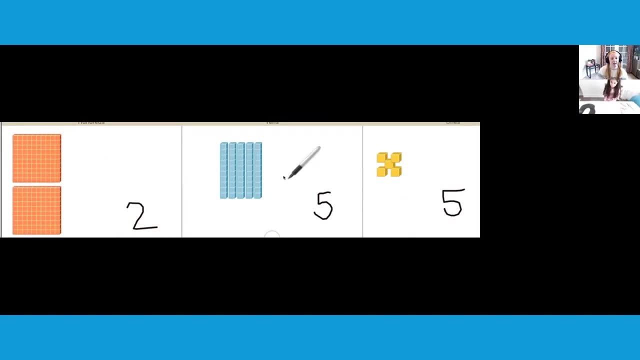 Can you do it? Yeah, where do we want to take away the one? Add it right here, Mm. hmm, Okay, thanks, Its name is Two hundred fifty-five. Good job, Nice work. That was a really good one. Shall we play a game. 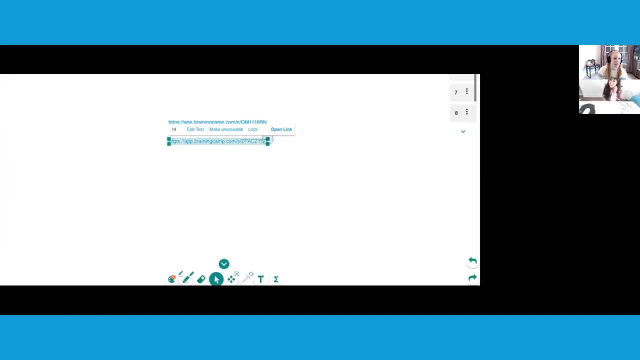 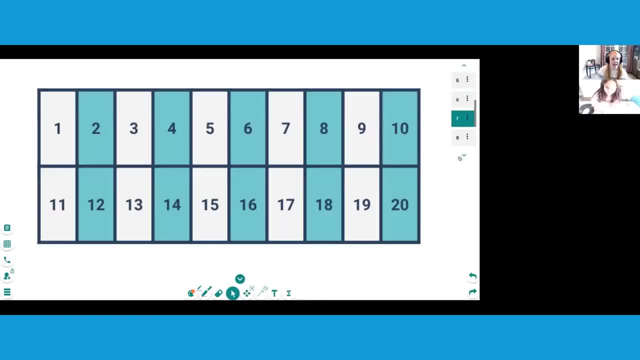 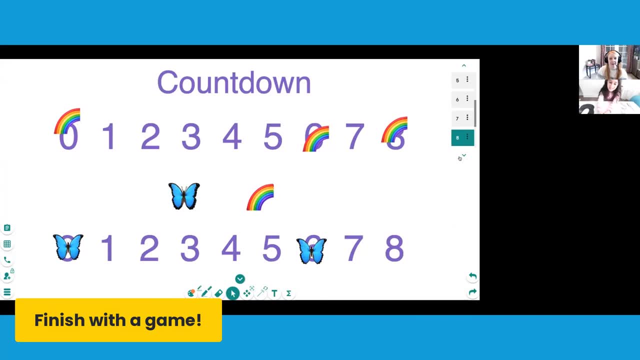 Shall we play a game? Let's play a game. Would you like to do guess my number, or shall we finish our countdown game? What about you decide today? Today? What? What about you decide today? Oh, is that okay? Can we finish the countdown game? 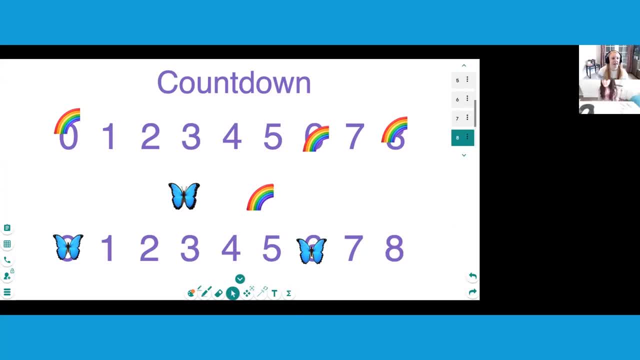 Sure, Because we didn't finish it before. So let's see, Let's keep Three points, Three points. Let's see what that is: Three plus one. Three plus one is More is four. Good job, Go ahead and move that rainbow to four.